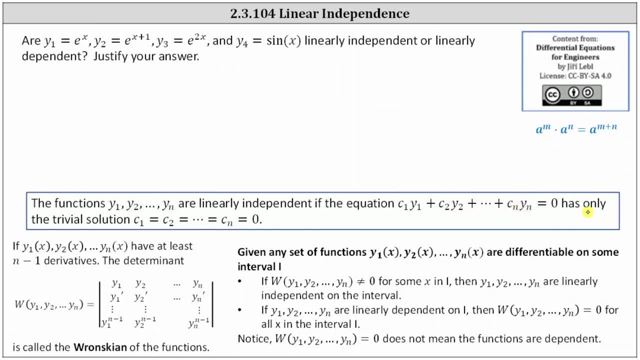 all the way down to plus c sub n times y sub n equals zero, has only the trivial solution: c sub one through c sub n equals zero, Which means if the functions y sub one through y sub four are linearly independent, then c sub one times e to the x. 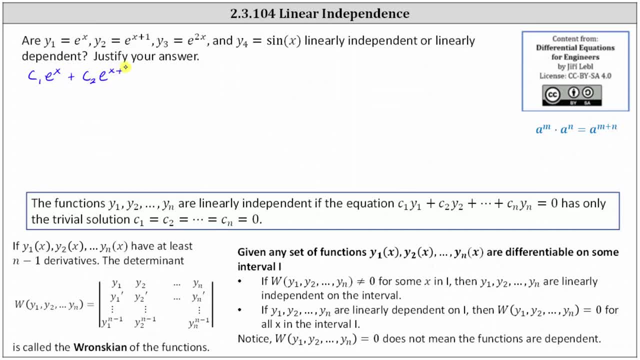 plus c sub two times e to the power of x plus one plus c sub three times e to the power of two. x plus c sub four times sine x equals zero only when c sub one through c sub four are equal to zero. If we can find any other solution, 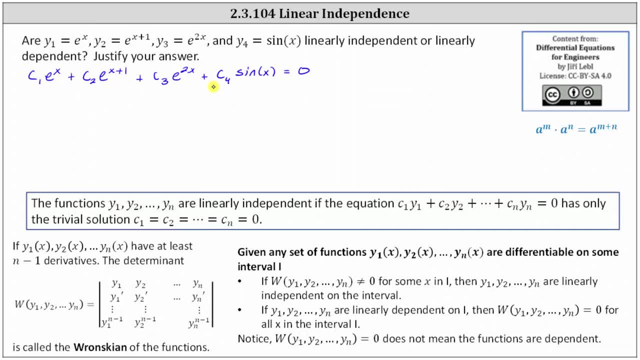 then the functions are linearly dependent. So, if we think that the functions are linearly independent, one way to show this would be to find the Wronskian shown below, which, in our case, because we have four functions, would be a four by four determinant. 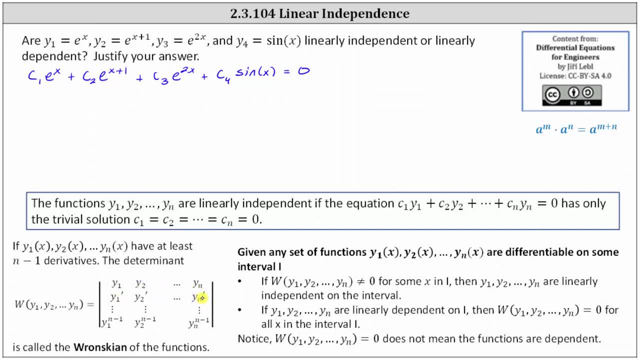 where the first row would be the given functions, the second row would be the first derivatives, the third row would be the second derivatives and the fourth row would be the third derivatives. Then we'd have to evaluate the determinant, and if the Wronskian doesn't equal zero, 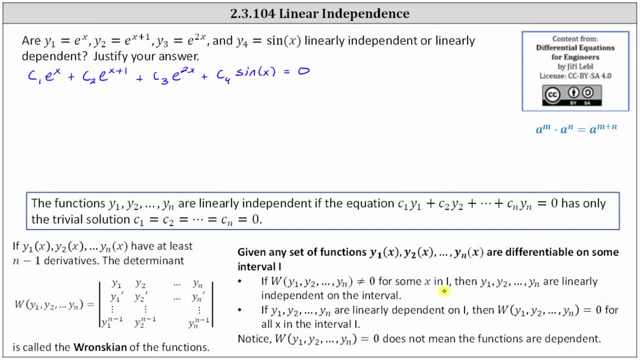 for some x in the interval, which in this case would be all real numbers, because the domain of all functions is all real numbers, then the functions are linearly independent. However, if we think that the functions are dependent, we simply have to find a non-trivial solution. 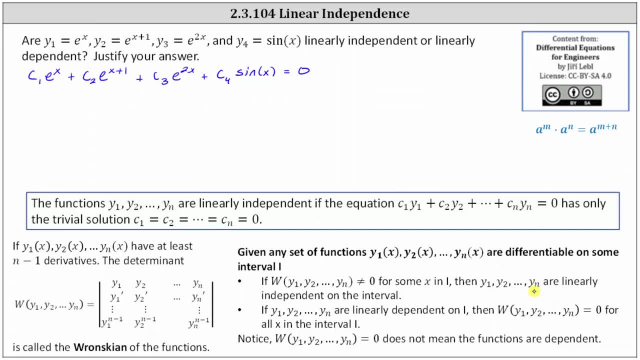 to the equation, So it's worth taking some time in analyzing the given functions. Using the exponent rule, a to the power of m times a to the power of n is equal to a to the power of m plus n. we should be able to recognize that e to the power of x. 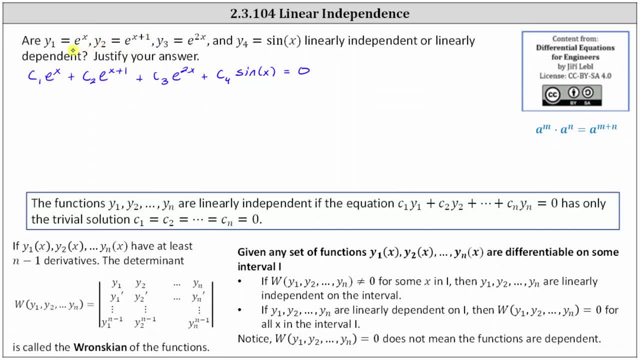 and e to the power of x plus one are scalar multiples of one another, which indicates y sub one and y sub two are linearly dependent and therefore y sub one through y sub four are also linearly dependent. To find the non-trivial solution: 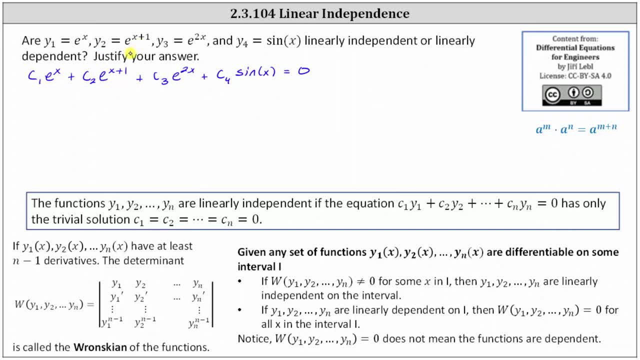 again, if we recognize y sub one and y sub two are linearly dependent, there must be some constant, which we'll call c. where c times e to the x must equal e to the power of x plus one. where c is some constant,